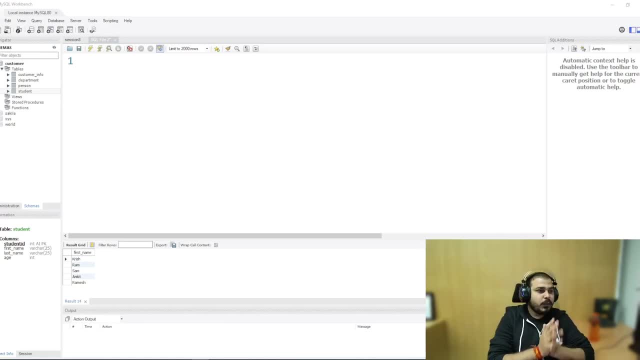 So, guys, we are going to continue the discussion with respect to MySQL and in this particular video, we are going to discuss about a very super important topic, that is, MySQL stored procedures. Now, stored procedure is a prepared SQL query that you can save so that the query 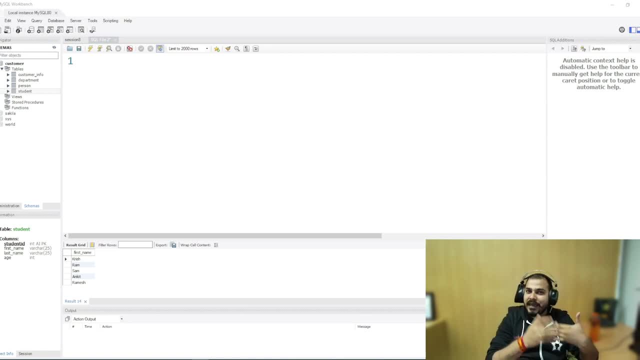 can be reused over and over again. That basically means it can be executed over and over again. Let's imagine that you have probably written some queries and in that specific queries you also provide parameters and you are going to execute it continuously and probably retrieving 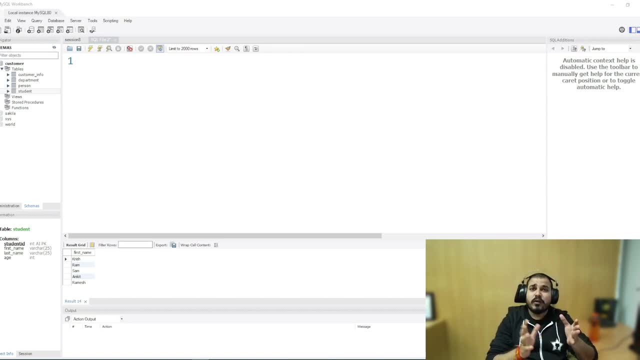 data. So in all this particular case, you can save that entire query in the form of stored procedure and you can execute it. Definitely it will help you to. you know, execute it quickly. You'll be able to see the output very fast soon right Over here in stored procedure you also have an 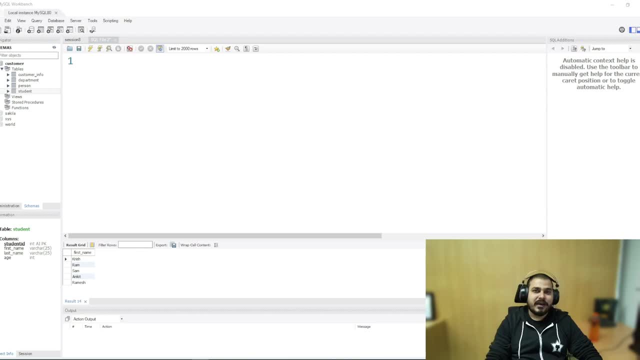 options to basically provide parameters also. take out the parameters also, like provide an input as a parameter, And also, if you want any kind of specific parameters, you can also take out the parameters also, like provide an input as a parameter, And also, if you want any kind of specific output, you can do that. Now let's go ahead and let's try. 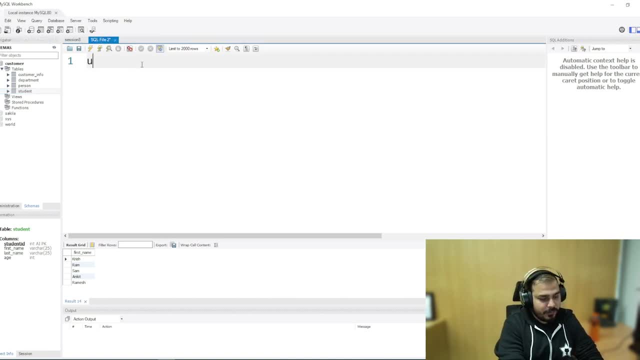 to see that, how a stored procedure is basically created. Now, first of all, what I'm going to do, I'm going to use my customer database And after this, let's see. I have some data like select start from student. Okay, So this is specifically my. you know the query. you can see where I have. 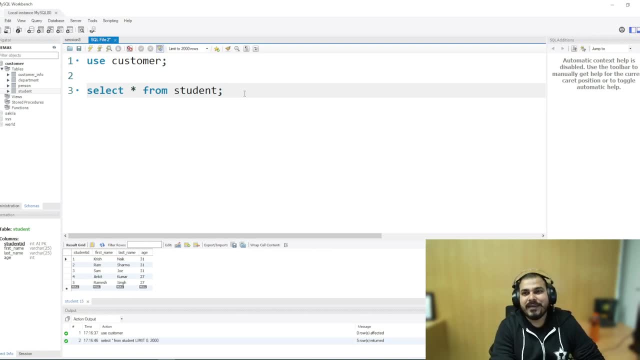 some amount of data over here. Now, what I can do is that let's say that I'm executing this small query again and again. Okay, select, start from student. Now let's see that I have some data over here. Okay, So this is basically my. you know the query. you can see where I have some data. 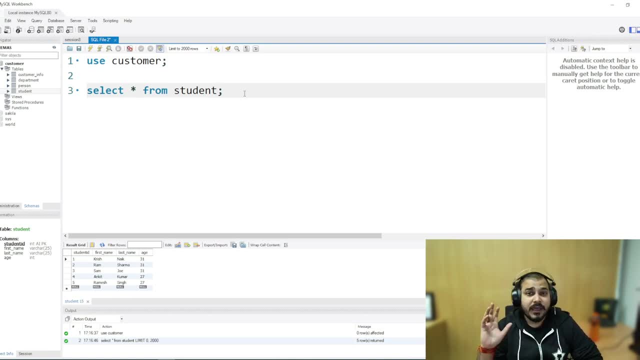 over here. Okay, So this is basically my. you know the query. you can see where I have some data from student. I'm just taking an example. you can write any kind of complex query in a stored procedure. Now suppose, if I want to create a stored procedure because I'm going to execute- 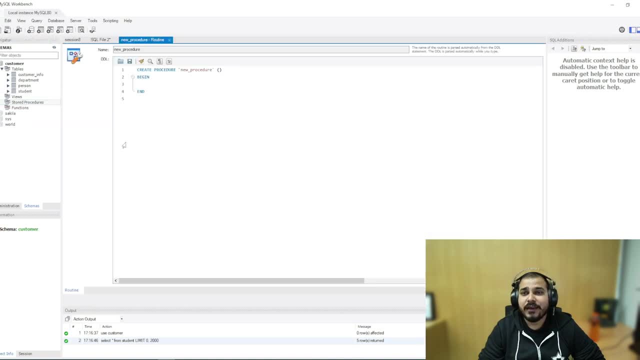 this query again and again. all I have to do go over here and just click on create stored procedure So you'll be able to see this one. And let's say that I'm naming this stored procedure as get student underscore info. So here you can see that this is how a stored procedure syntax is. 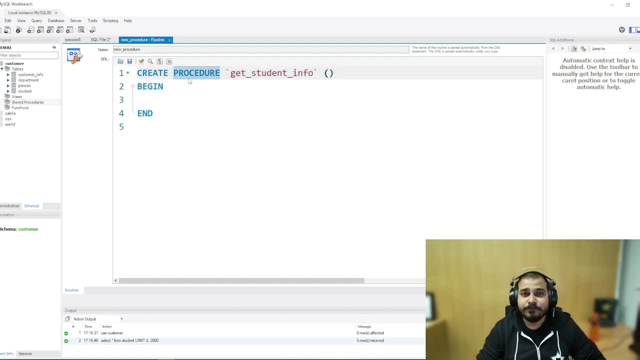 how you can basically create it. you use a create procedure, create procedure- keyword. along with that, you give the procedure name And then whatever query you're going to execute again and again, you'll basically write inside this. So over here I'll. 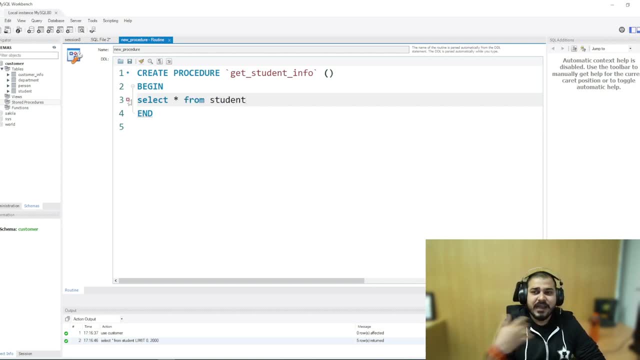 say select start from student. let's say that I'm just going to execute this query And probably I want to create this particular- I have named this particular- stored procedure: get student underscore info. Okay, So after this, this is how you basically create it. right now I'm not giving 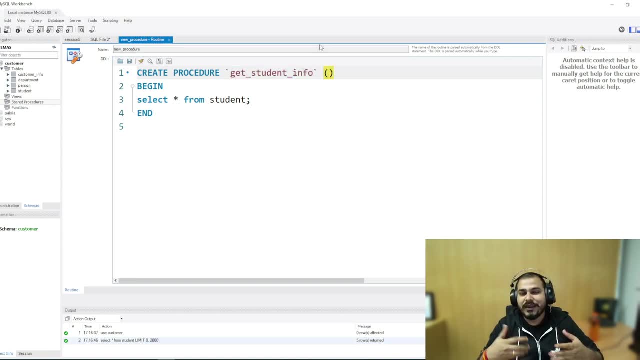 any kind of input parameters. Later on I'll also show you how you can create a stored procedure. You can give input parameters and probably see it, Okay. So now what I'm going to do? I'm just going to apply it. So here you'll be getting an option of applying and then just execute this SQL query, Okay? so once you create this here, you can now see that a stored procedure has actually been created. get. 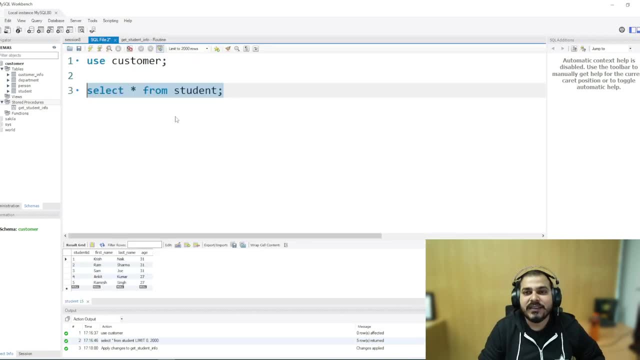 underscore: student underscore info. Now the next thing, in order to execute this, all you have to do is that just write call, call function and then you basically call: get student underscore info Right. So when you probably give this and just execute it, you will be able to see that I'm able to see all the data from the students, right, select start from students. So here you can definitely see all the values that you're able to get it over here. So this is how simple a stored procedure is right. So just have to use the call keyword and just write the stored procedure name and then you'll be able to get it. Now let me do one thing. let me just go and make some changes over here. Now, what I'm going to do over here is that suppose let's consider the 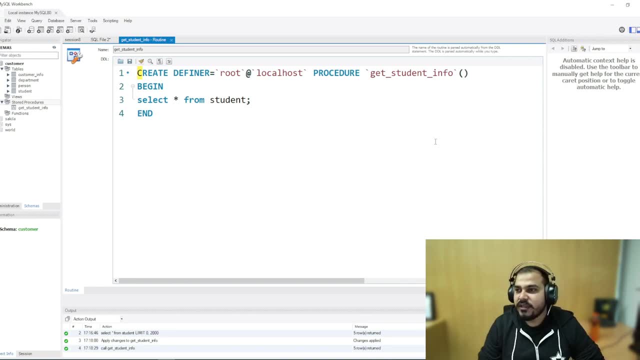 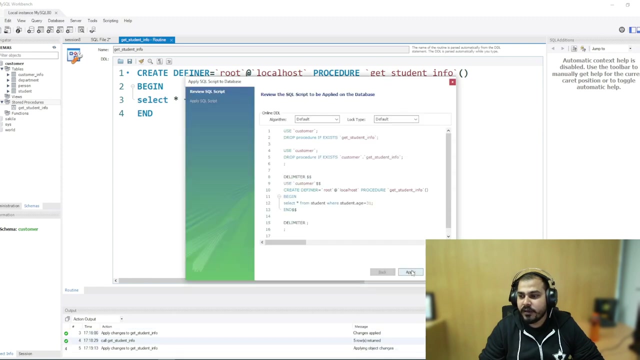 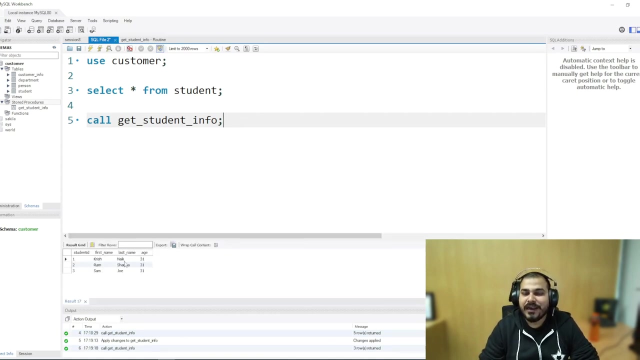 that I'm going to give some kind of parameters. Okay, So in this particular case, let's say that I'm going to give a parameter like select star from student, where student dot age is equal to some values like 31.. Okay, so I'm just going to execute it. Okay, let's see what will happen. Now I'm going to go back over here and just execute this thing. Now, here you can see that my entire query is getting executed, because that entire query I've put it inside my stored procedure. 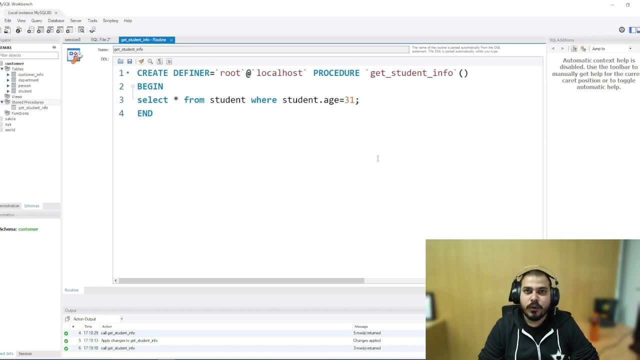 One condition that I had written: my age should be 31.. Now can I give an option where I can make the stored procedure parameterized, you know? so I just give my input from here And based on that, it takes the input over here. So in order to define the input, there are various ways. one is in, out, And you can also use the combination of in, out. Okay, First of all I'll just show you with the help of in, Okay. so here I'm going to basically use in. Let's consider that I'm using in. you can also write it in capital letter, And then I'm going to give my parameter. 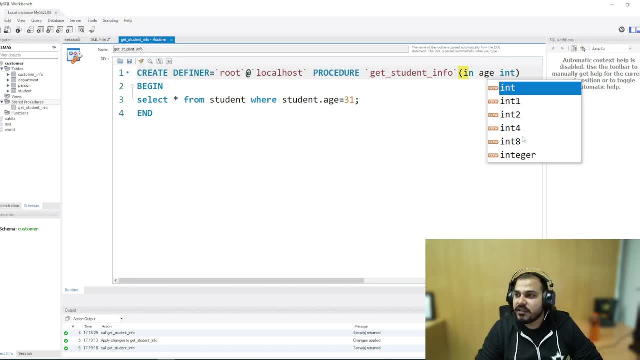 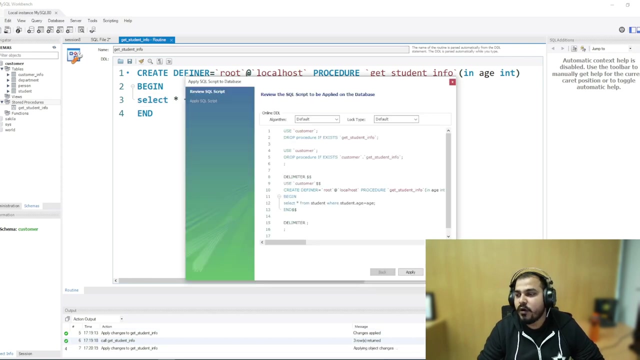 Name and my data type name. That's it. So this is the parameter name that I'm actually going to give over here And I'm going to just replace it over here. So this basically says that whatever parameter I'm giving over here when I'm calling this particular stored procedure, get underscore student, underscore info. this will be given over here And, based on that, I will be able to retrieve the student's name. Okay, the entire information of the student. So now let me go ahead and execute this very quickly. So this has got executed And now. 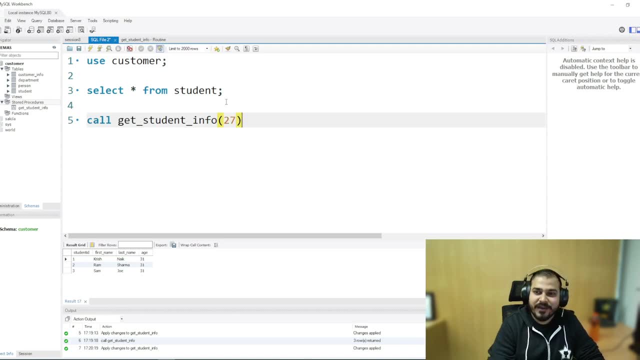 let me make some changes Now. here I'm basically going to say 27.. Galaxy select star- it's just like I'm calling this particular stored procedure with the input parameter 27.. So once I see this here, you can see that I'm having people with the 27 age. So there is specifically that specific record I'm actually getting. What we have done over here is that we have just parameterized, So here I've also given 31.. You can also see the records as 31.. So this was one type what you can actually do in order to create parameterized things right. 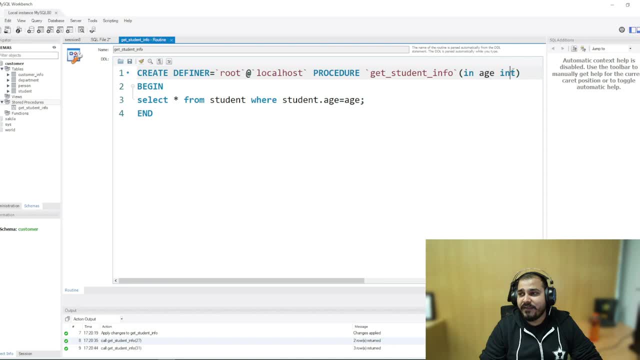 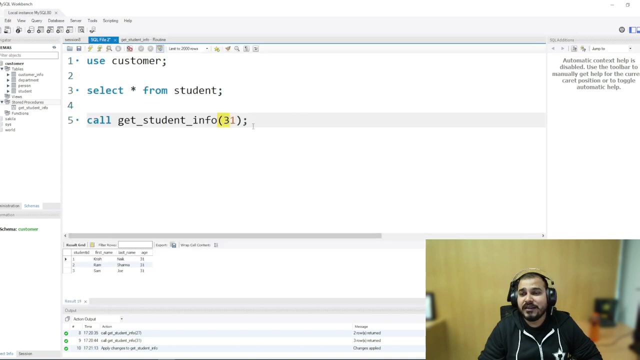 You can also give anything like: if this variable is a varchar, you can give varchar with that specific number of parameters. But always remember, if I remove this student dot age, okay. instead I just write: age is equal to age because age is also a column inside my student table right. So if I execute this, this will definitely not get executed because it will get confused. where it is basically identifying with. it is not able to identify the student age column and the age column. 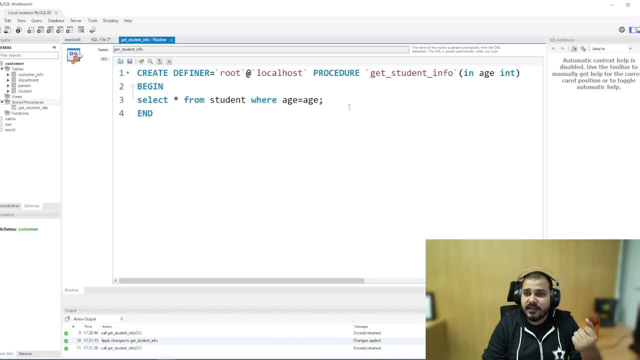 The age parameter that is coming in. That is the reason what I have done is that I have written as student dot age: Okay, so student dot age is specifically saying that the student table column age is getting compared to that particular input parameter that I'm actually giving So till here. I think you have, you know this right Now, and this is quite easy: input parameters. Now, what is the main use of the output parameters? Let's see this. So, guys, till now we have discussed about the in keyword. 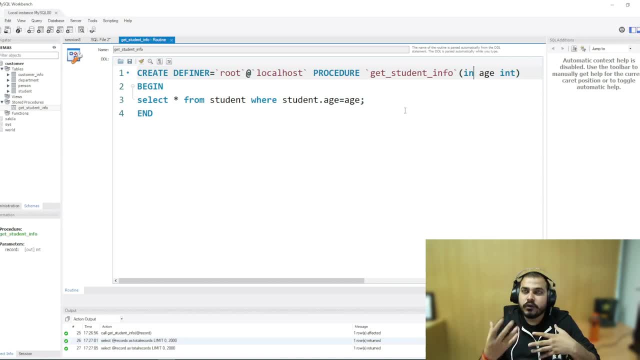 Now let's say that probably I want to execute a stored procedure and return some value, Okay, and then we can basically see that particular value. So in this particular case, I will just make some changes in the stored procedure. First of all, I will basically use out keyword that is going to give the output, that what we are specifically returning from this particular stored procedure, Okay, so here I'm just going to say that output records. Okay, so this is the records that is getting returned. 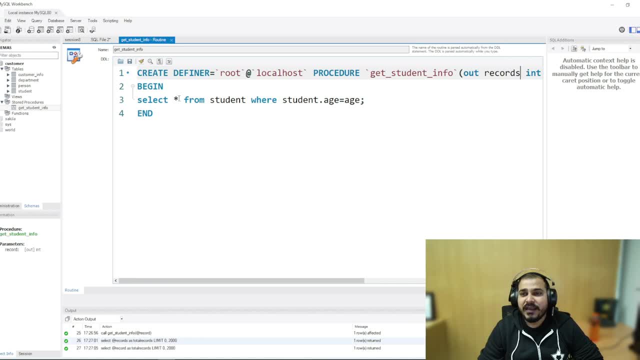 Now this record can be my total number of records, So I'll write select count star from student where student age is equal to. since I'm not providing any parameter over here, I can write 31.. So obviously I know that how many number of records will be there? three records will be there, So let's execute this. Now what is going to happen is that when I execute this, still one thing is basically missing: how I will link this records with this count, right? So for this I'm going to say that I'm going to use out keyword. 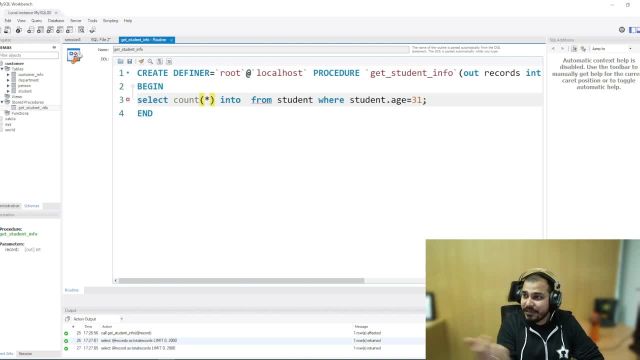 that what I'm going to write. I'm just going to set select count star into this records variable and this record variable get returns from this particular stored procedure, which will have the condition as student dot age is equal to 31. so I'm just going to apply it. so once I apply it over, 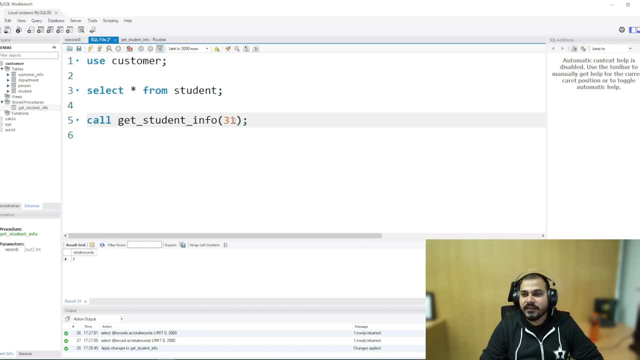 here you will be able to see this now. let's go and execute now. here, two changes will be there. first of all, I will give one parameter which will basically return the result right. whatever result is basically coming from there, from that stored procedure, it will get stored in this. and then, if 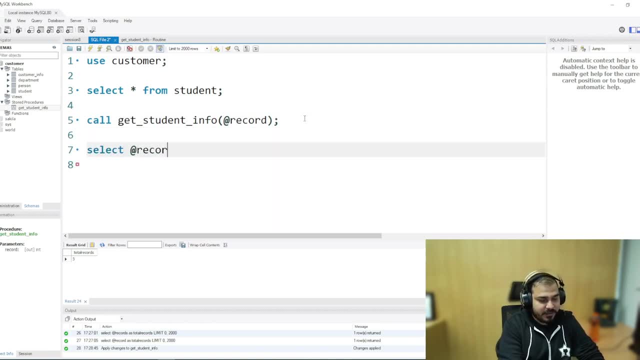 I want to basically display this. I can write select at the rate record as total record. okay, so once I execute both of this, this should give me the answer. let's see. so I'll execute this. and finally, you can see that the total number of records is three. let me make it to 27 because 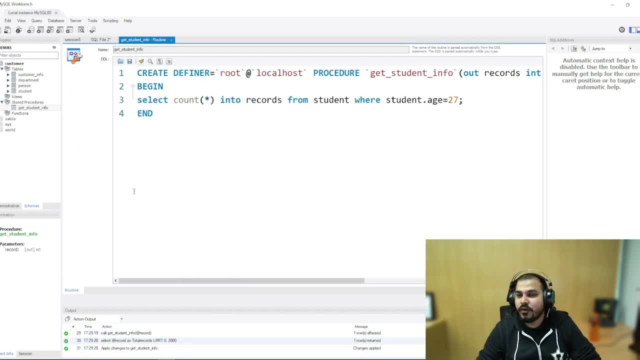 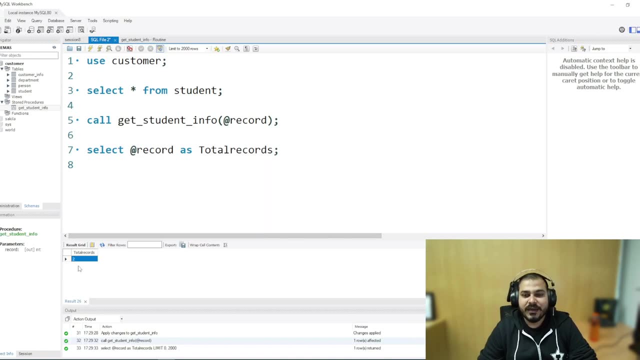 in this particular case, I will be able to get two records, okay, just to show you whether this is getting executed or not. right? so over here you can definitely see that I'm getting two records. so this is some examples with respect to in and out. sorry, out and in or in and out. now one assignment that I would like to give you. try to combine in.